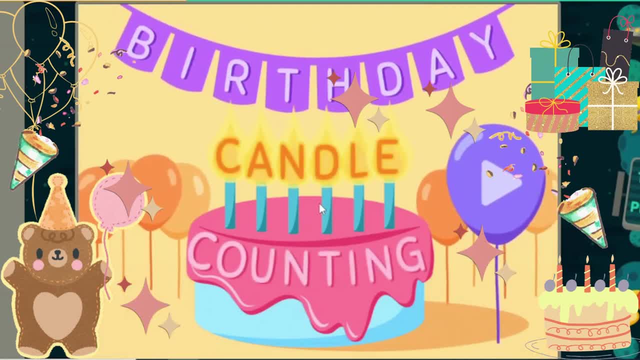 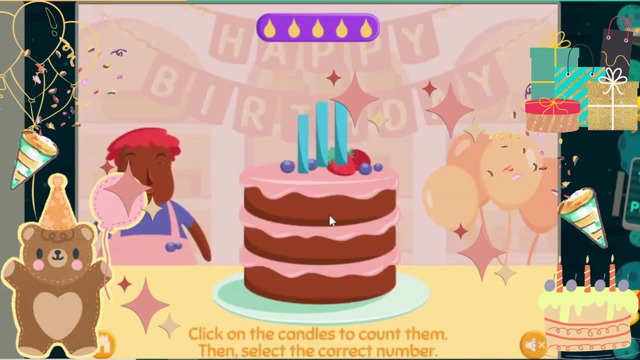 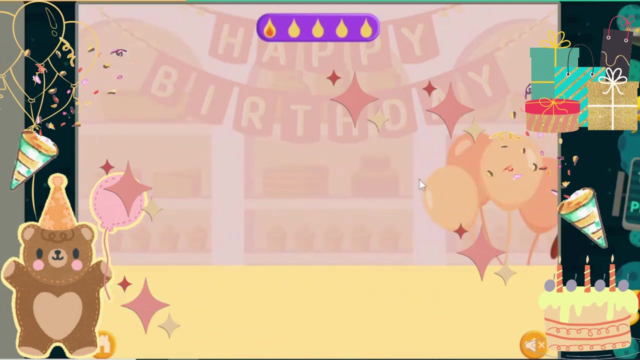 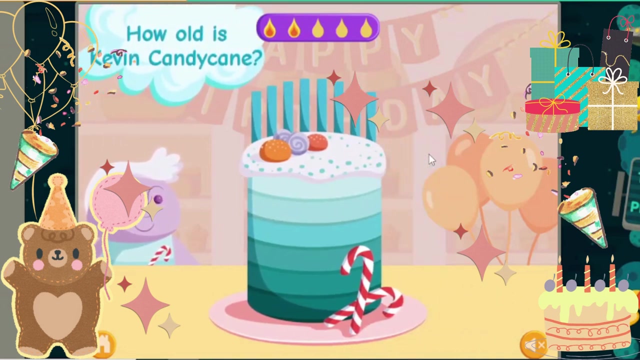 Birthday Candle Counting. Click on the candles to count them, Then select the correct number. How old is Billy Blueberry? One, Two, Three, Three. How old is Molly Macaron? One, Two. How old is Kevin Candy Cane? One, Two, Three, Four. 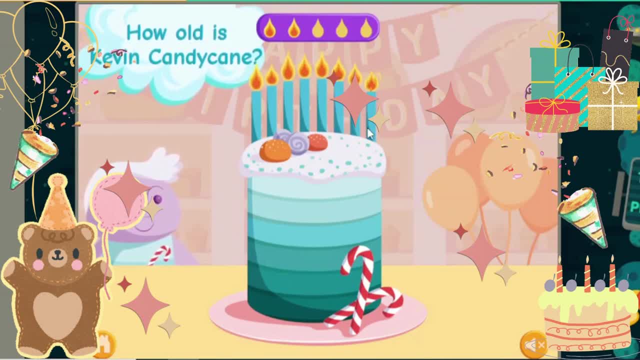 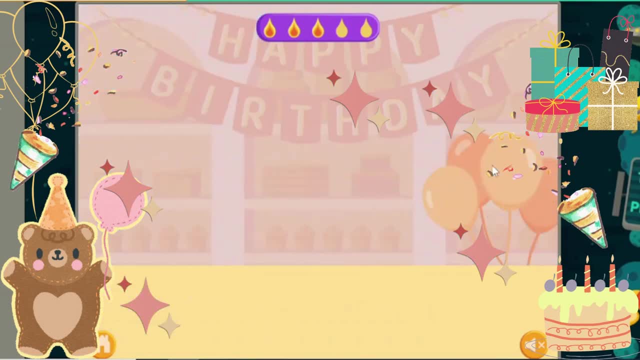 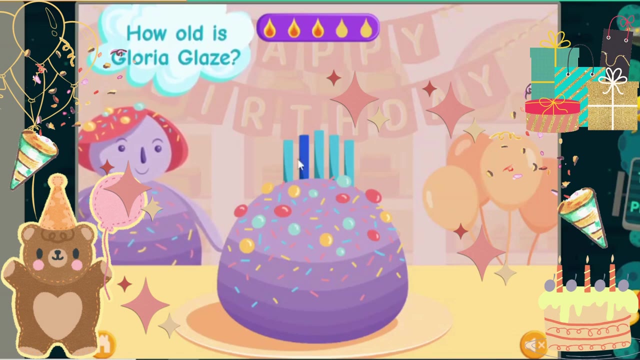 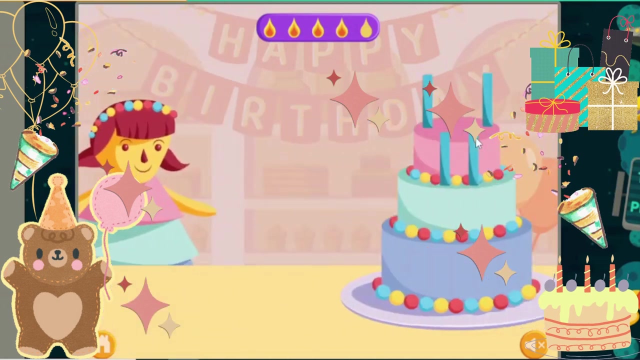 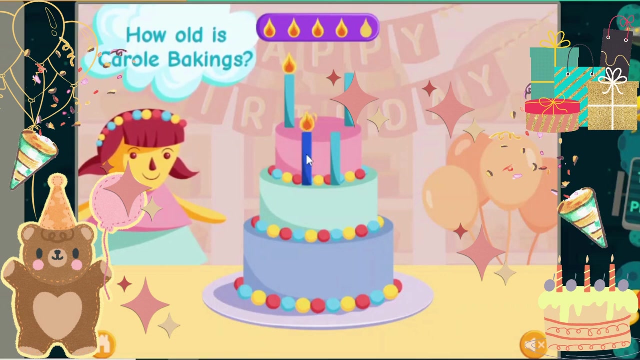 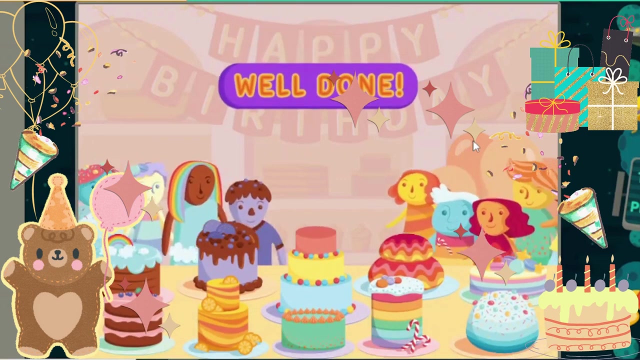 Five, Six, Seven, Eight. How old is Gloria Glaze? One, Two, Three, Four, Five, And how old is Carol Bakings? How old is Carol Bakings? One, Two, Three, Four, Five, Six, Seven, Eight, Nine, Ten, Eleven, Twelve, Thirteen, Four, Four, Five, Six, Seven, Eight? 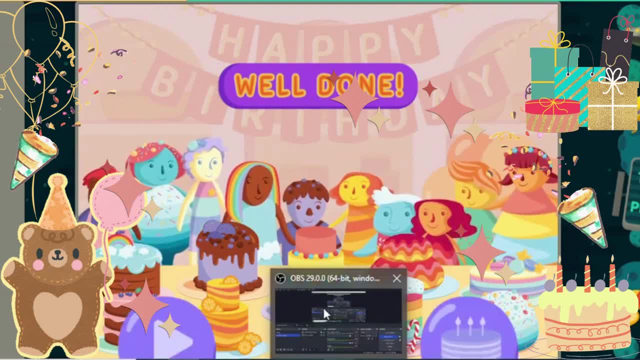 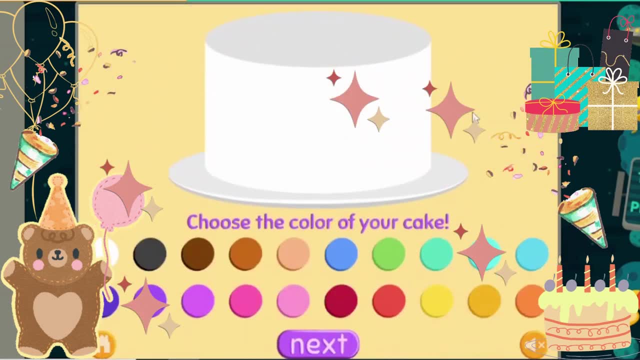 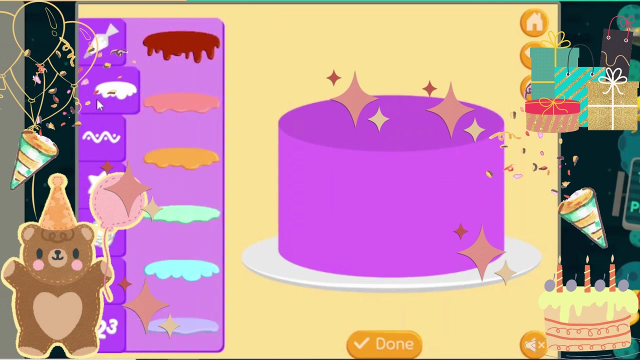 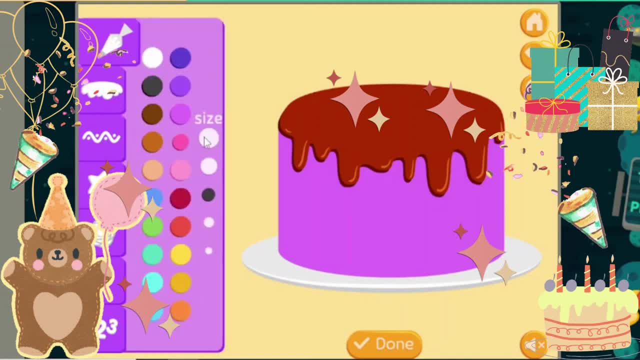 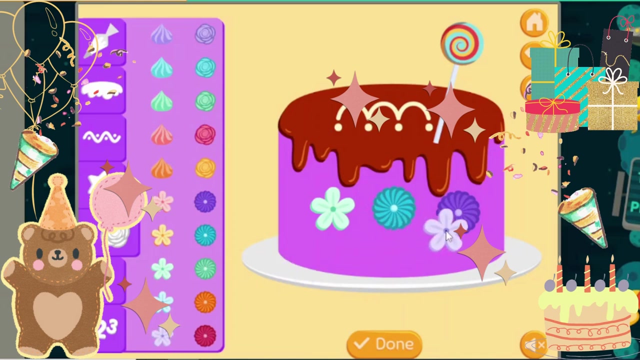 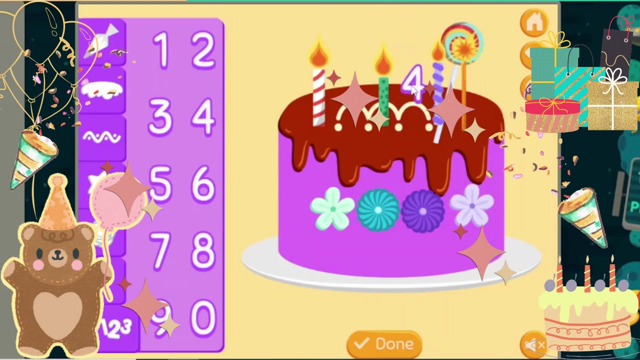 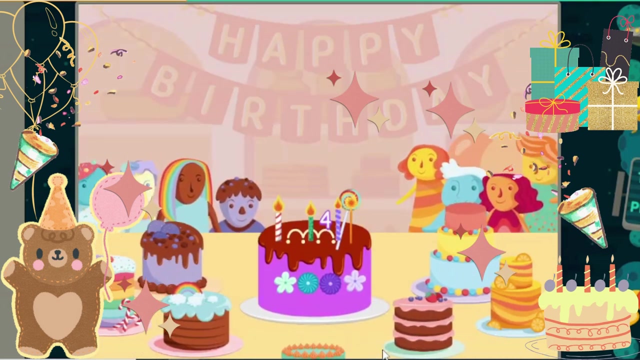 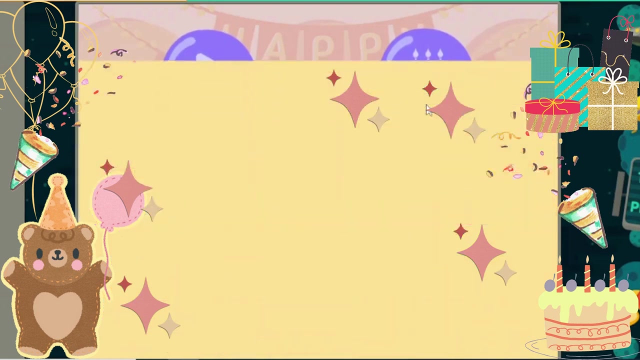 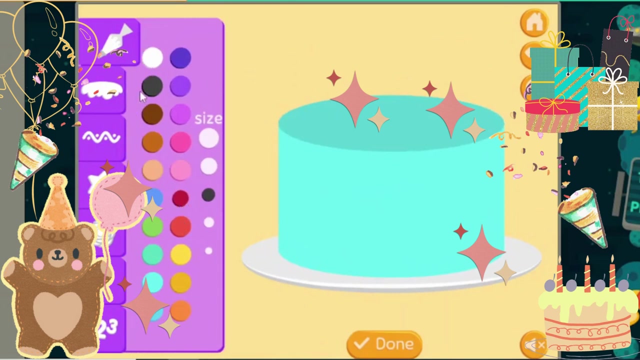 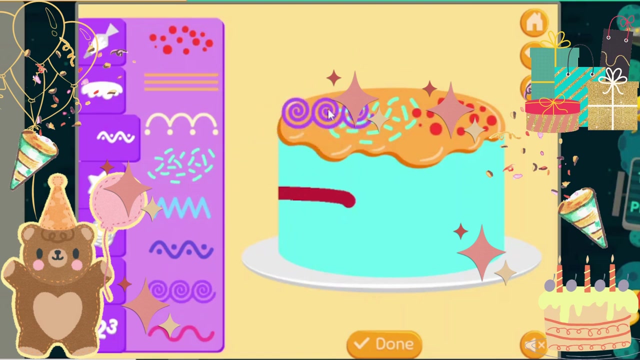 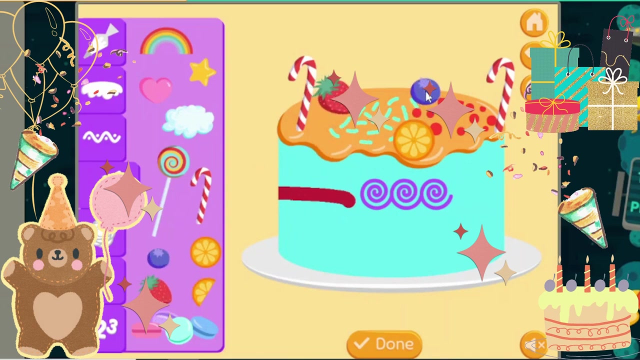 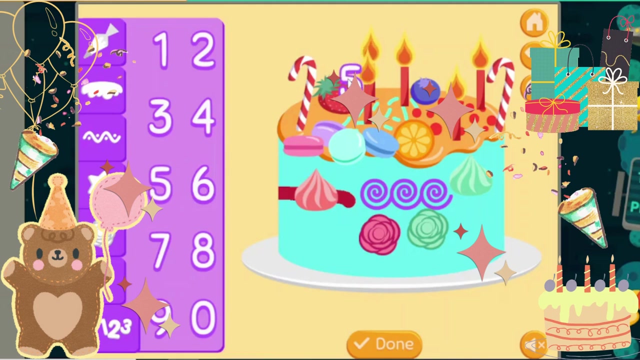 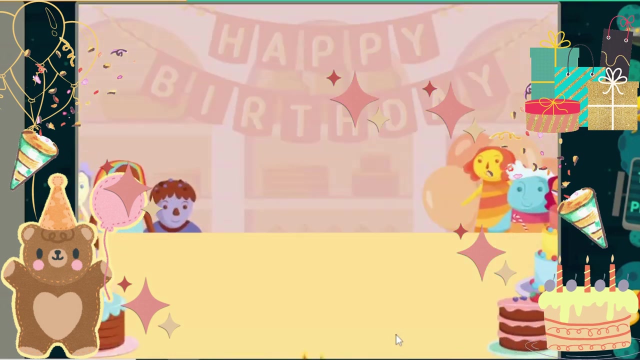 Thirteen, Thirteen, Thirteen, Thirteen, Thirteen, Thirteen, Thirteen. Thank you, Thank you, Thank you. Do you want to play again or decorate your own cake? Thank you, Thank you, Thank you. Do you want to play again or decorate your own cake? 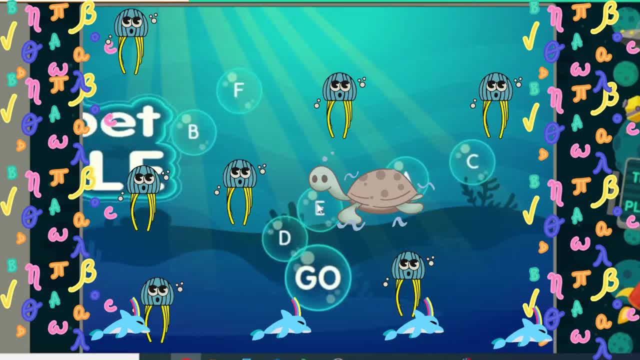 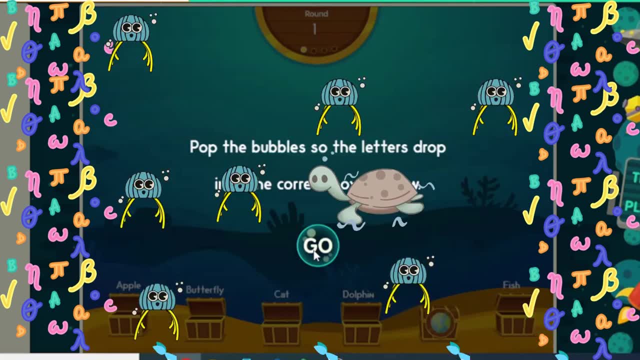 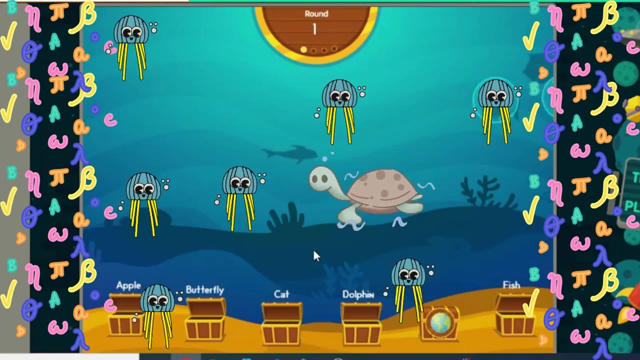 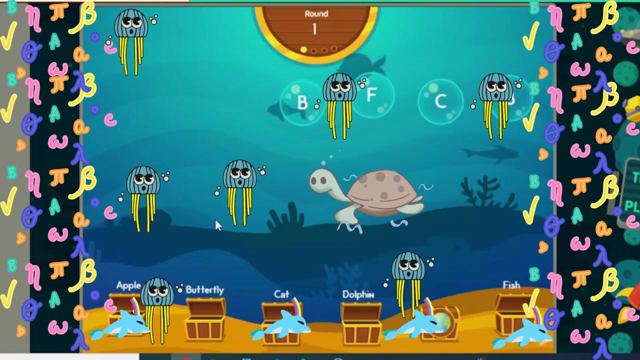 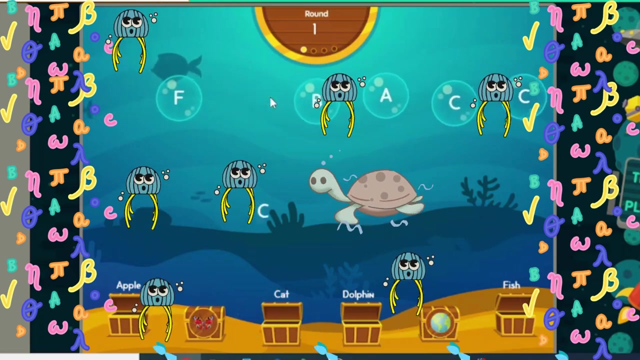 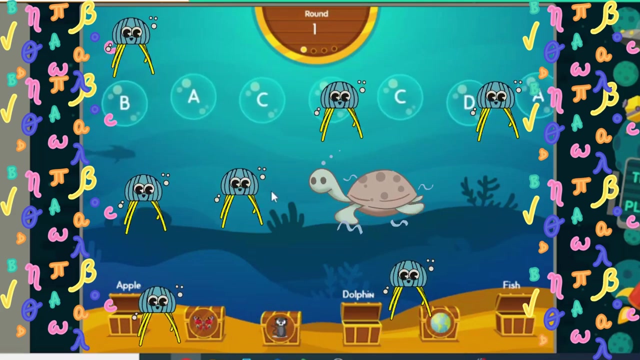 Do you want to play again or decorate your own cake? Alphabet bubble. Pop the bubbles so the letters drop into the correct boxes below. Pop the bubbles so the letters drop into the correct boxes below. Pop the bubbles so the letters drop into the correct boxes below. 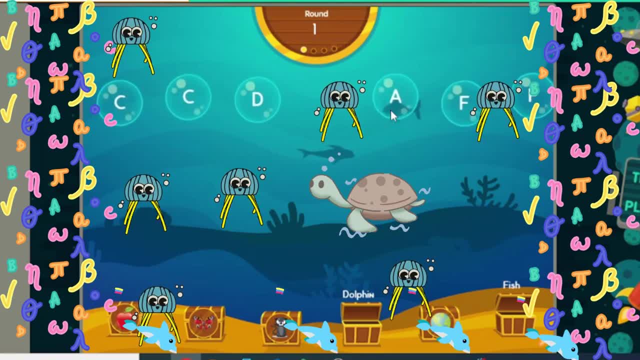 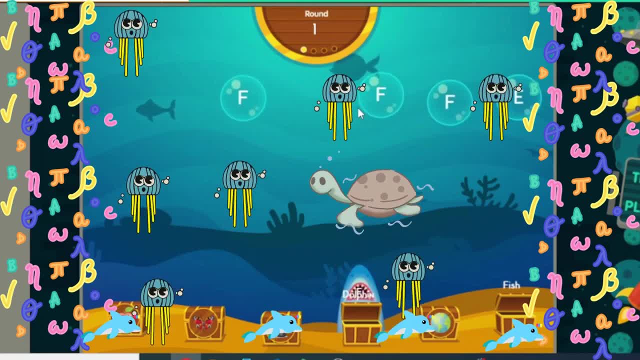 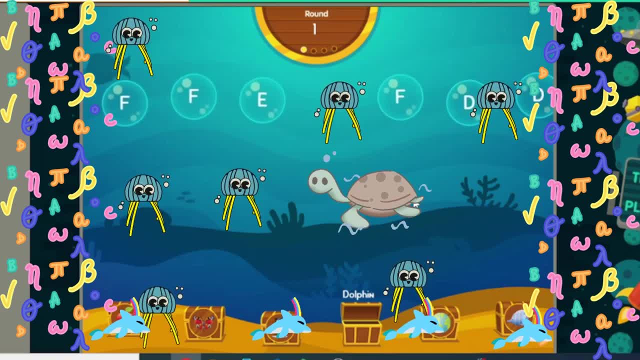 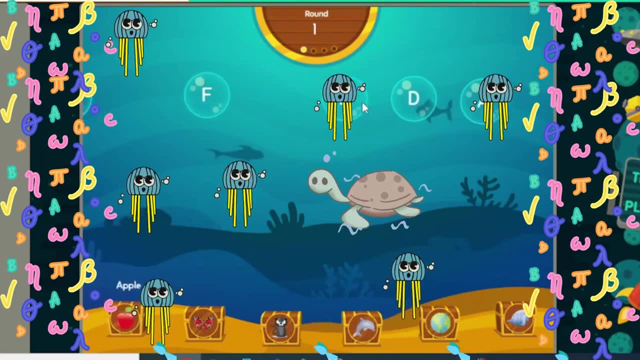 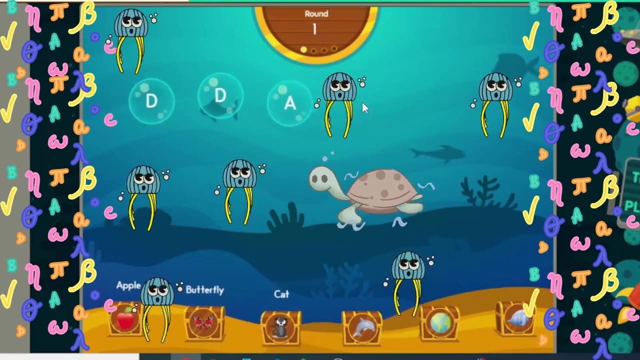 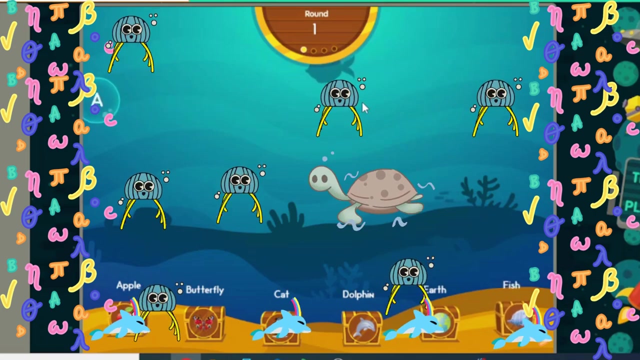 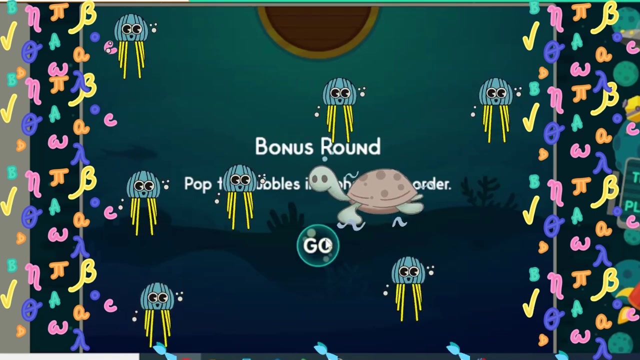 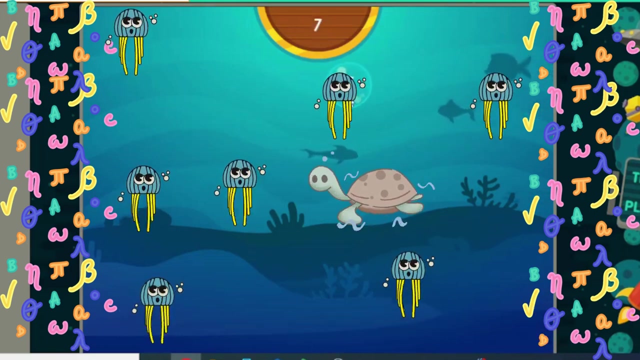 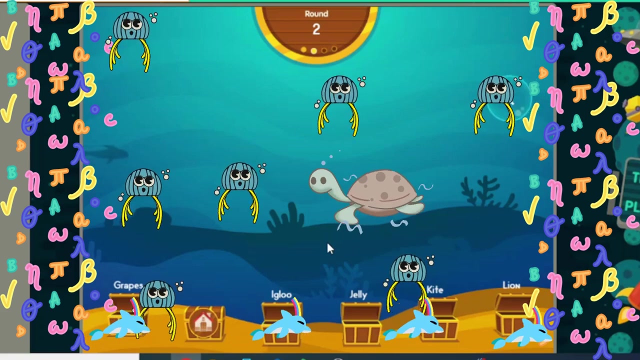 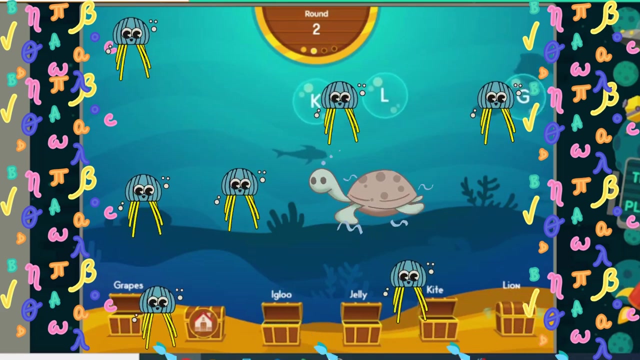 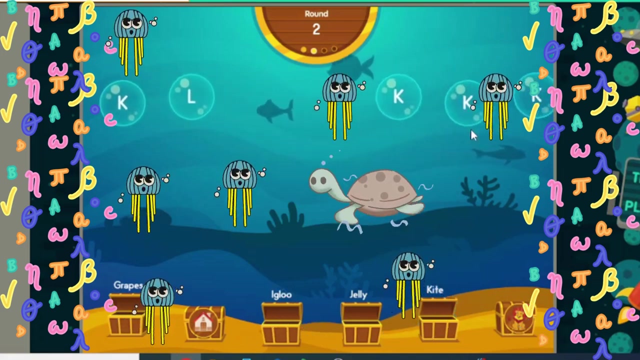 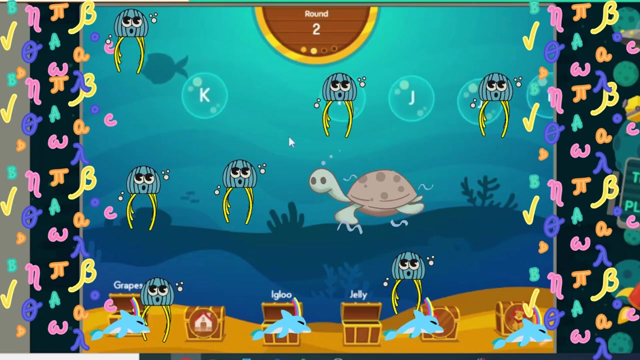 A, Apple B, Butterfly C, Cat D, Dolphin E, Earth F, Fish, Nice, Pop the bubbles in alphabetical order. Awesome, You did it in seven, 3-4.. Okay, let's try not to miss anything. 2-1.. 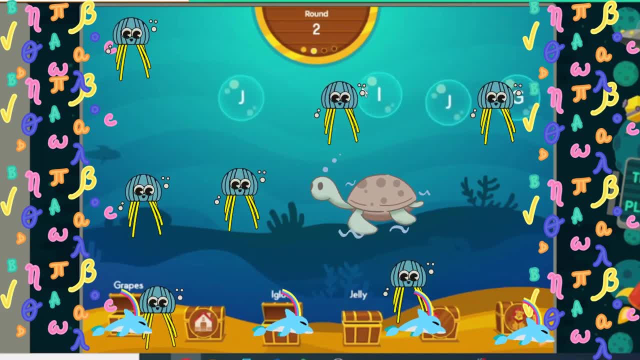 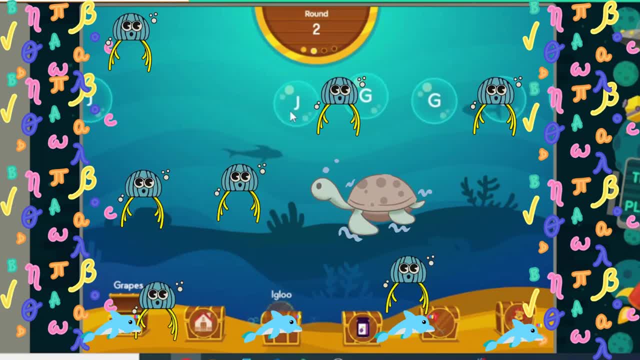 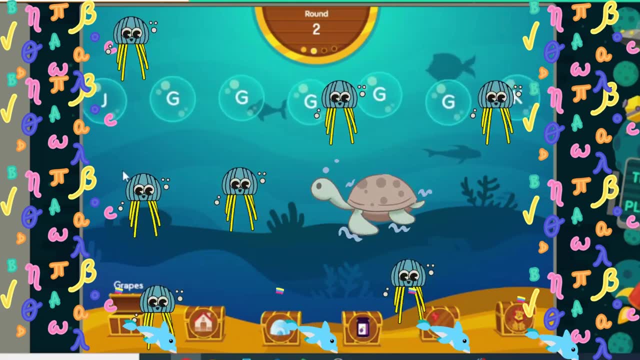 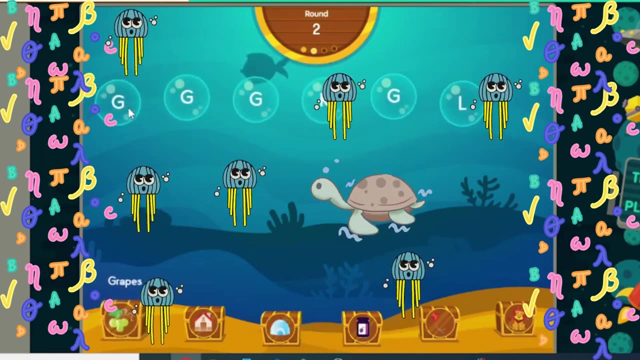 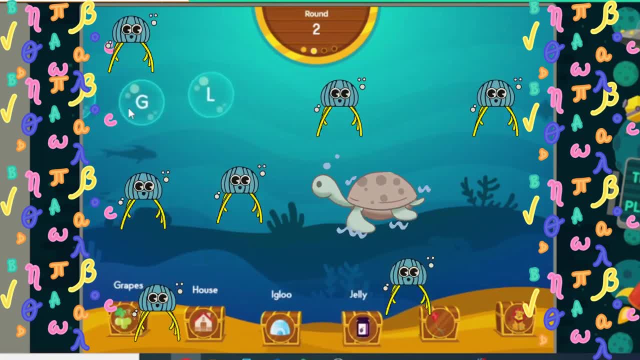 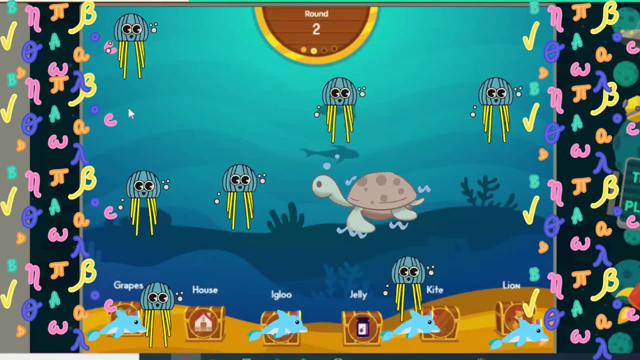 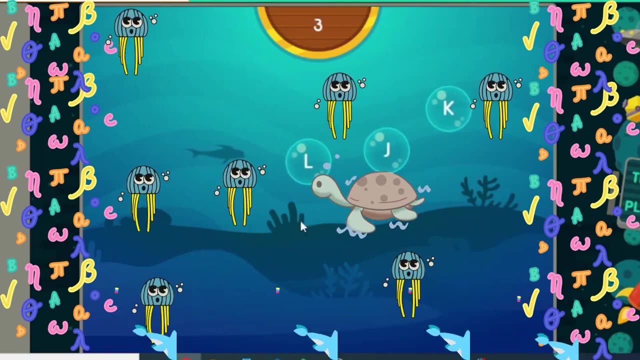 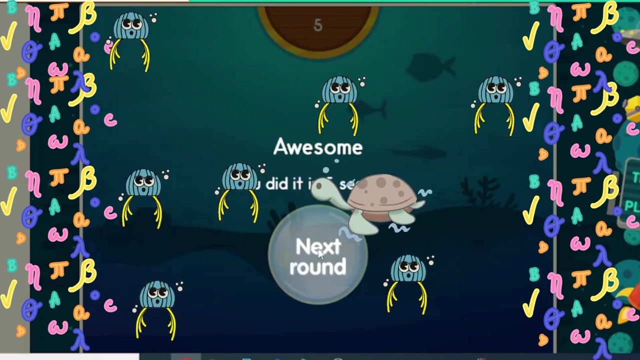 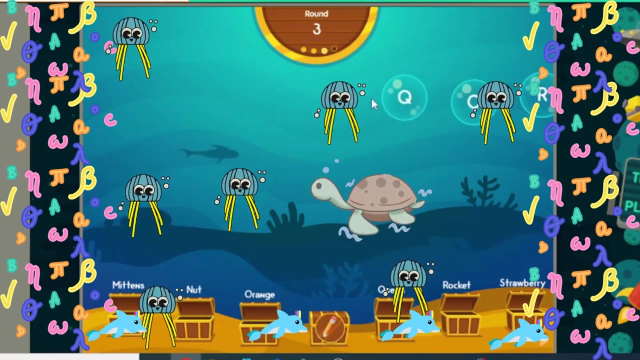 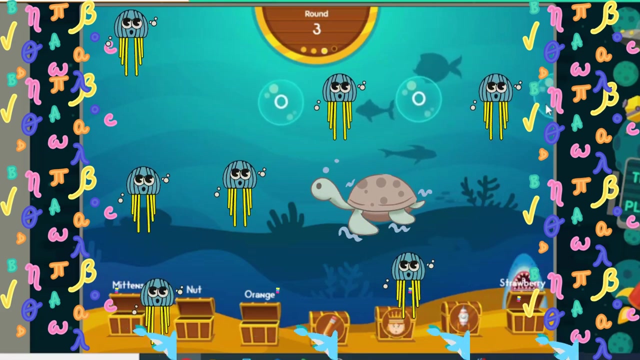 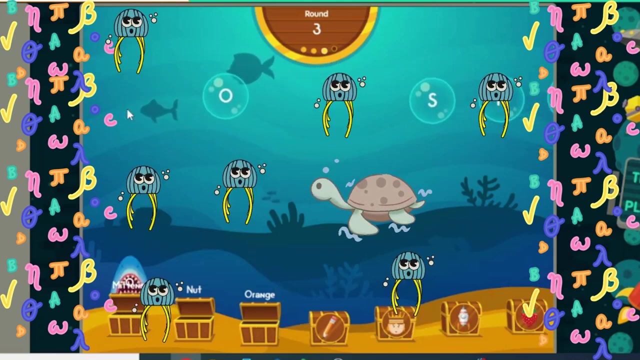 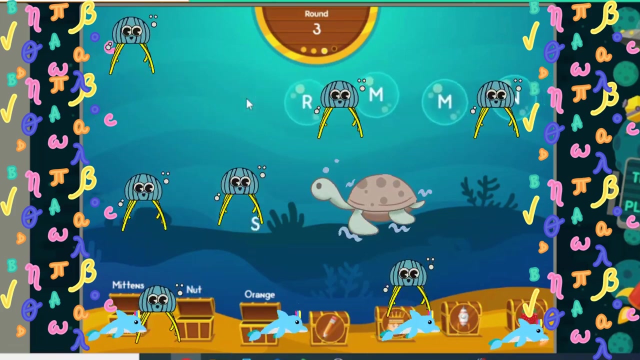 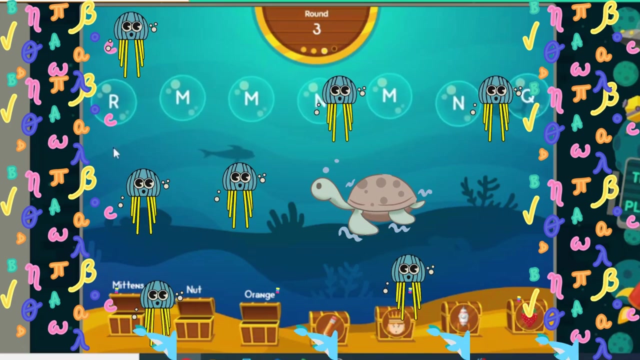 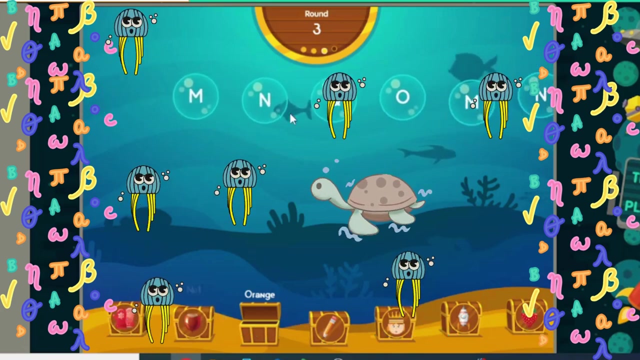 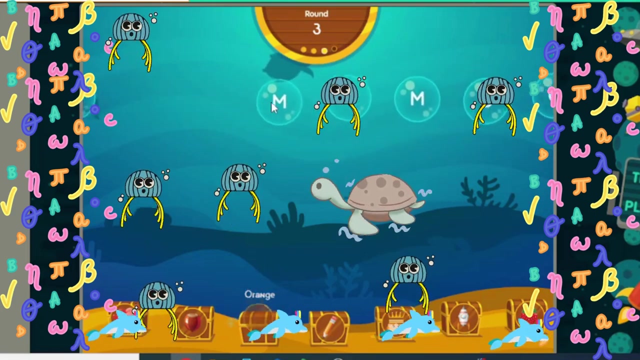 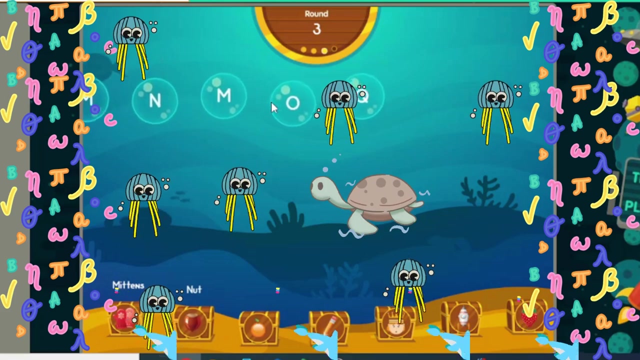 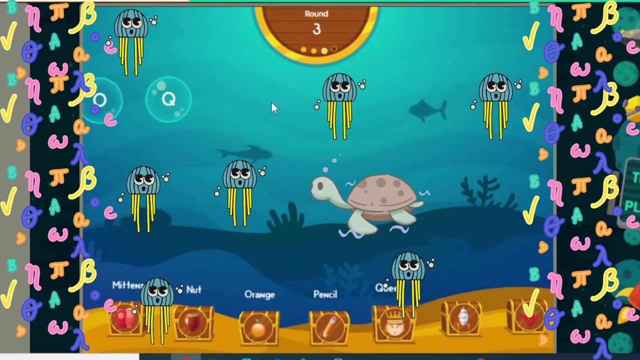 J, Jelly, K, Kite, L, Lion. Good job. Pop the bubbles in alphabetical order: Awesome, You did it in 5 seconds. M, Mittens, N, Nut O, Orange P, Pencil, Q, Queen R, Rocket S, Strawberry. 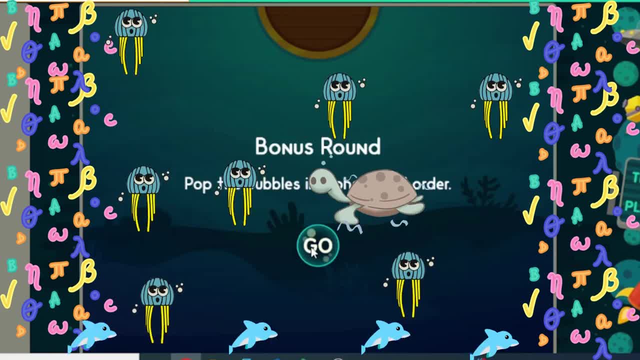 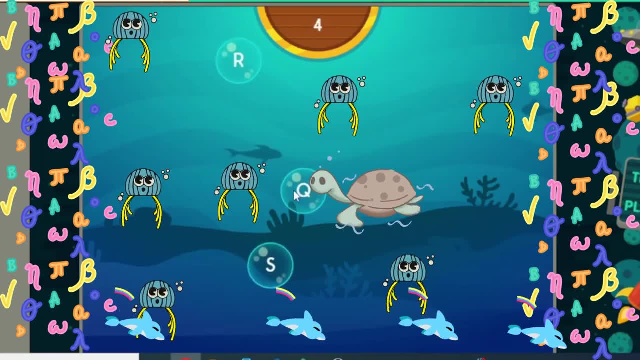 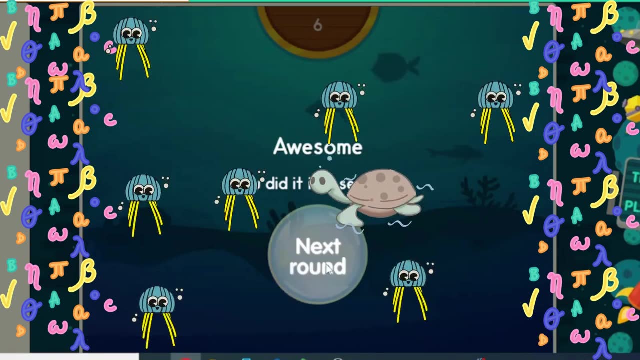 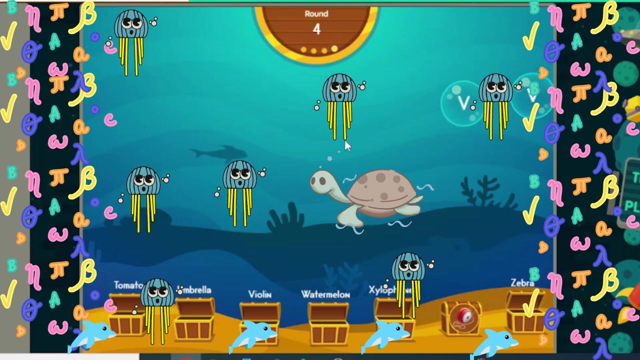 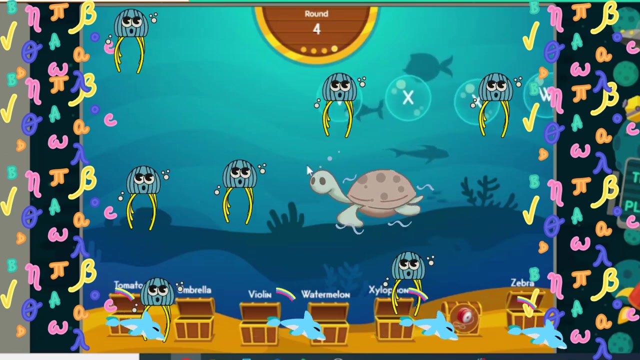 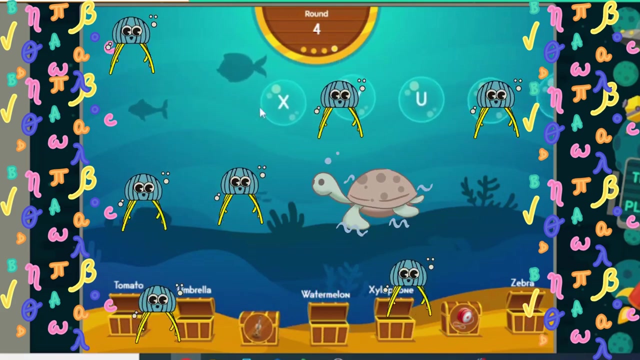 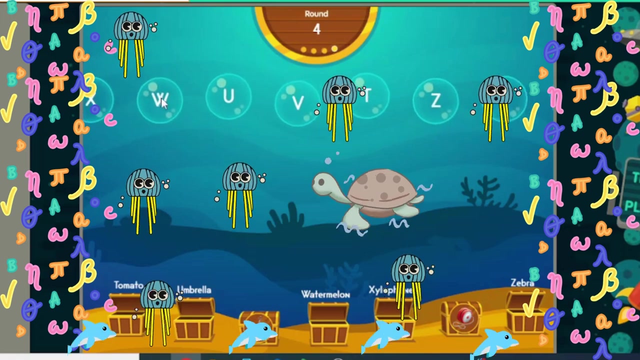 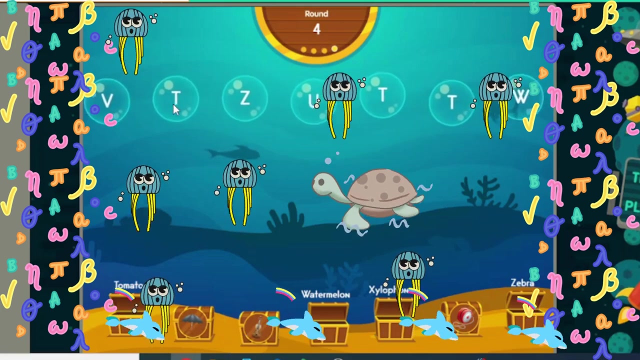 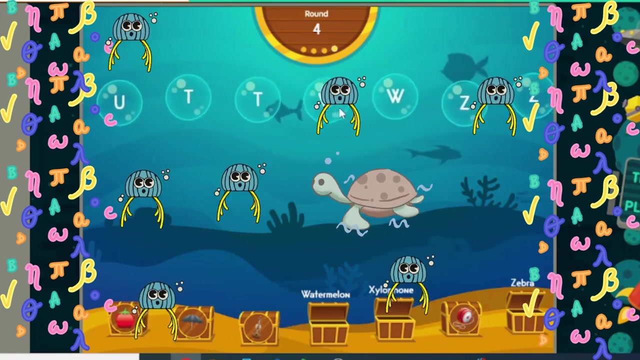 Nice Pop the bubbles in alphabetical order: Awesome, You did it in 6 seconds. Good job, You did it in 6 seconds. M Grapes, I Grapes O Kite. M Montage S Balloon, O Balloon. 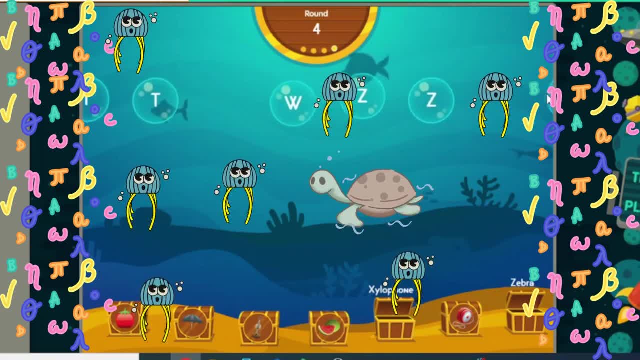 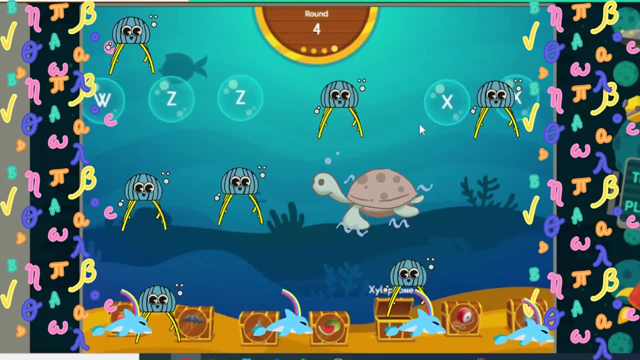 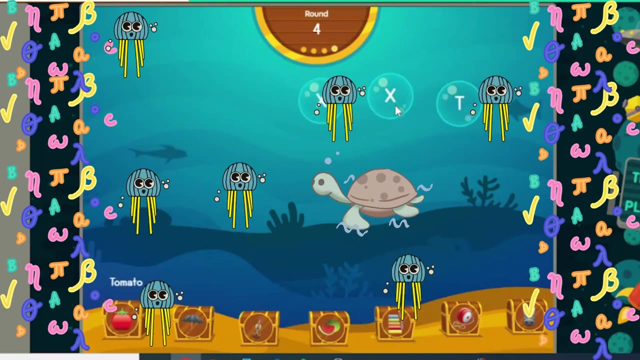 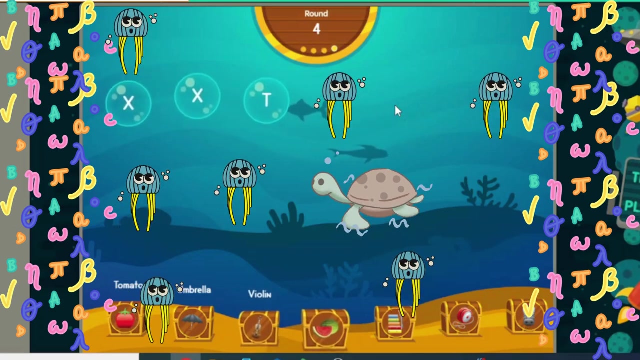 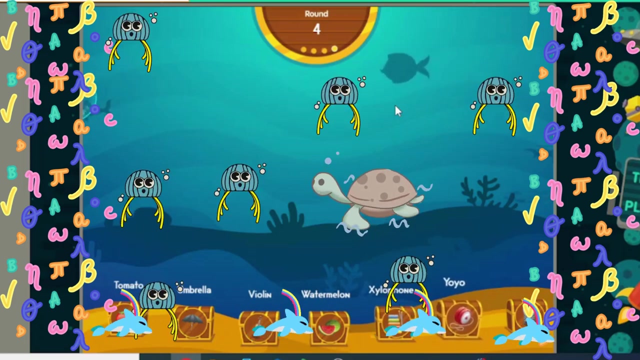 M Mastiff O Balloon O Balloon M. Mastiff O Balloon M. Mastiff O Balloon T Tomato U Umbrella, V Violin, W, Watermelon, X Xylophone Y Yo-Yo Z Zebra.